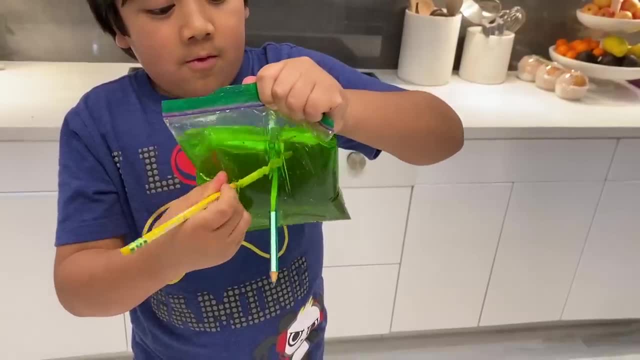 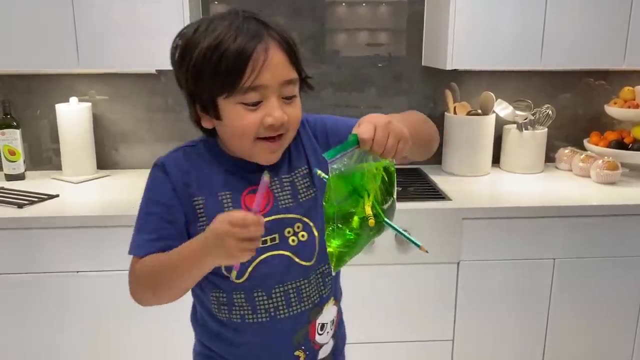 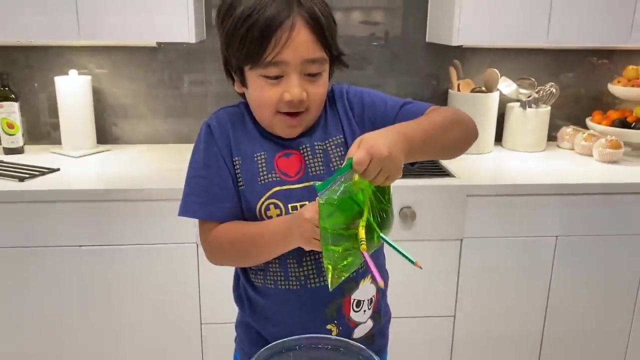 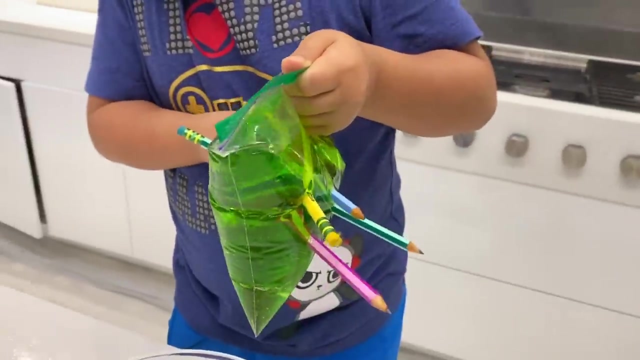 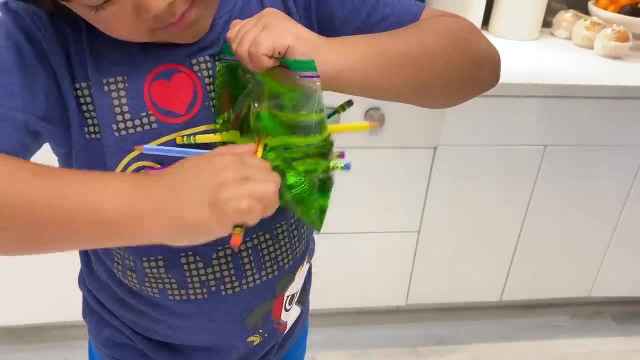 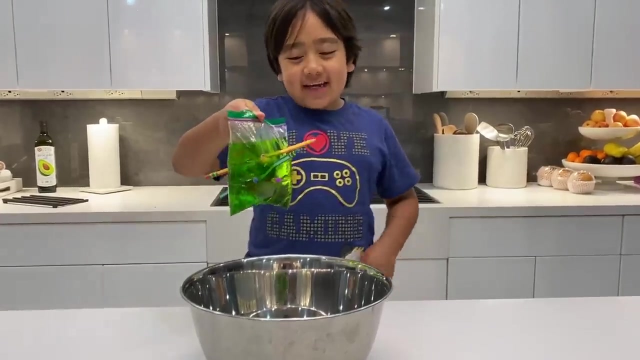 Like: Like this Got another one. Here's pencil number three, Like that: Yeah, All right, guys. pencil number four: Are you ready? Okay. And then the last pencil number five, Like that: Perfect. And here's the fun part: Taking out all the pencils. Whoa, Whoa, Whoa. 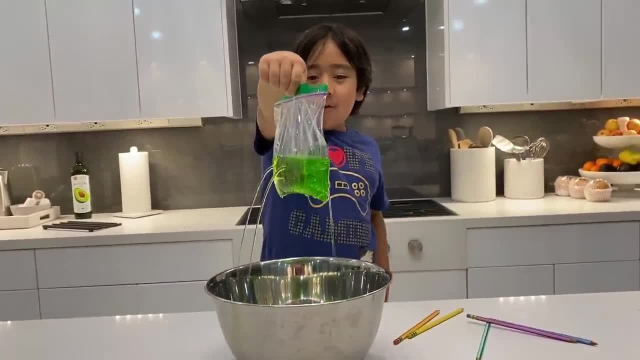 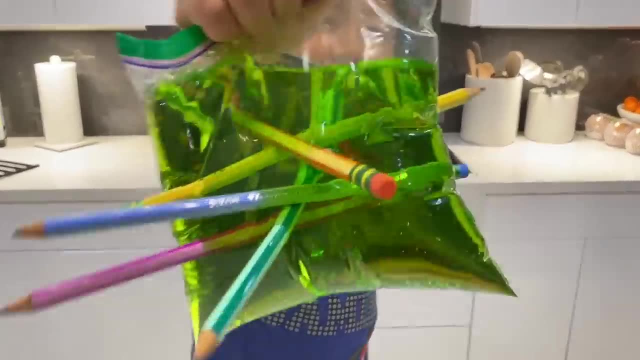 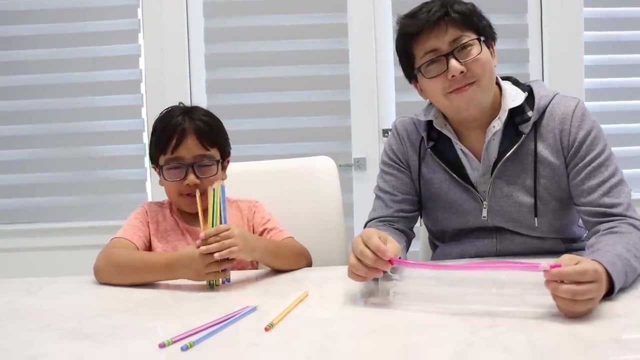 All the pencils are out. Look at this. All right, guys, let me show you guys how I do the big version. Welcome to Ryan's World. Hi guys, Today we're going to do a science experiment with pencils And we're going to 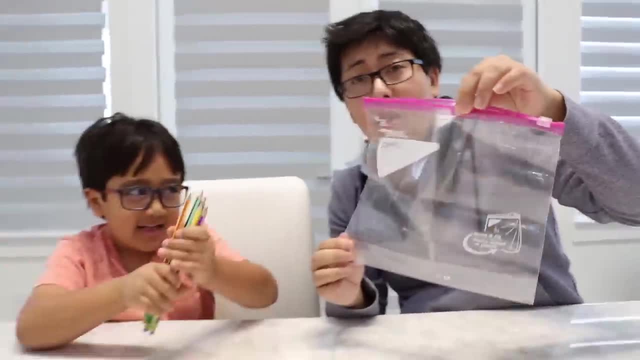 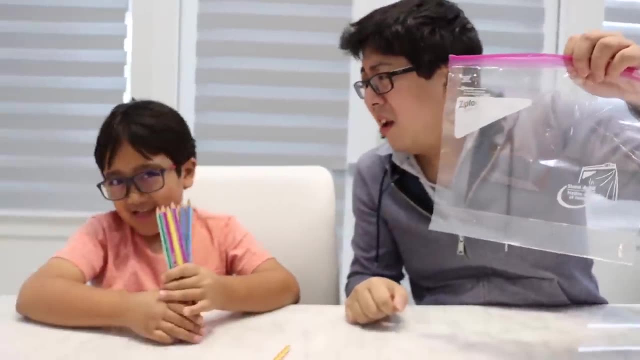 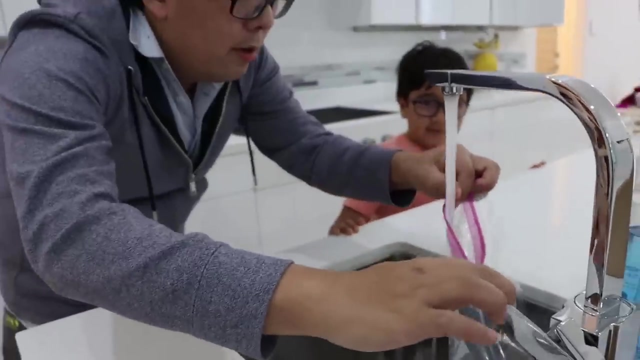 poke these pencils through a Ziploc bag And the Ziploc bag will have water inside it. Whoa, Whoa, Ryan. that means all the water is going to leak through. Ryan, That's the choose bag. First, let's put water inside the bag. Okay, let's fill it up. Hopefully, Ryan's telling me a truth, because 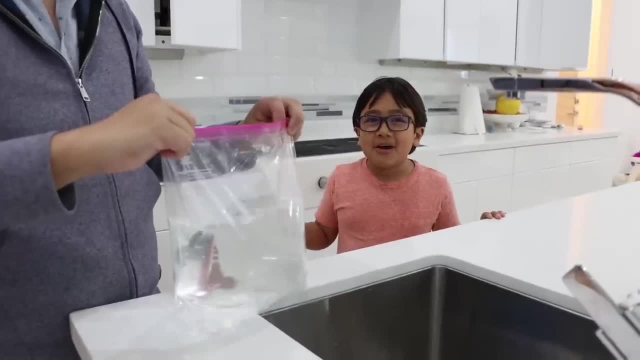 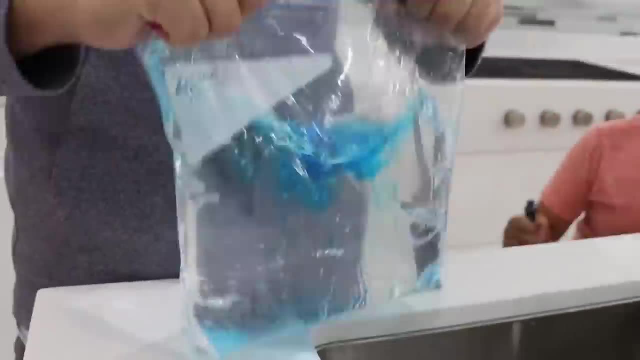 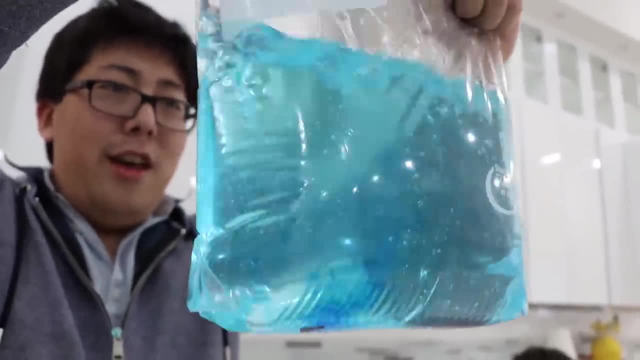 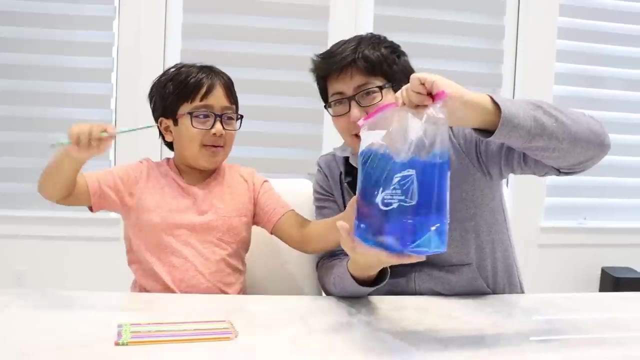 Well, look at the color- Ah nice. Look at the ocean Next up. we're gonna need a sharpened pencil. Don't forget to ask your grown up for help. All right, here we go, We're gonna poke it through. 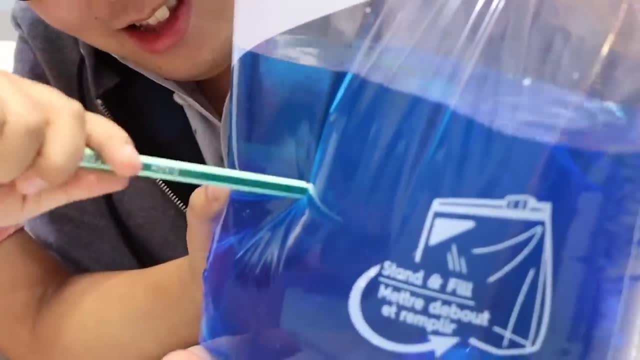 Three, two, one. Is it gonna work? Yeah, it's not gonna make a mess. Oh, it's poking through. Whoa, whoa, whoa, It's poking through, Whoa. Look the pencil's inside. 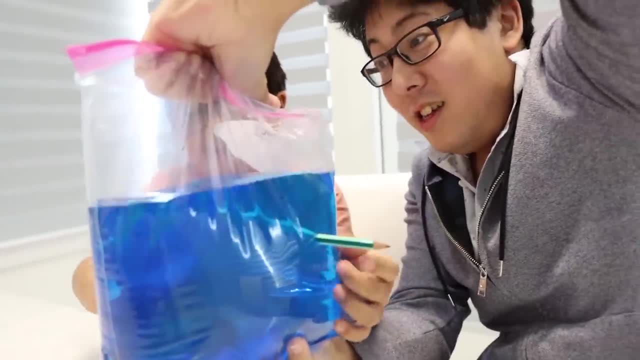 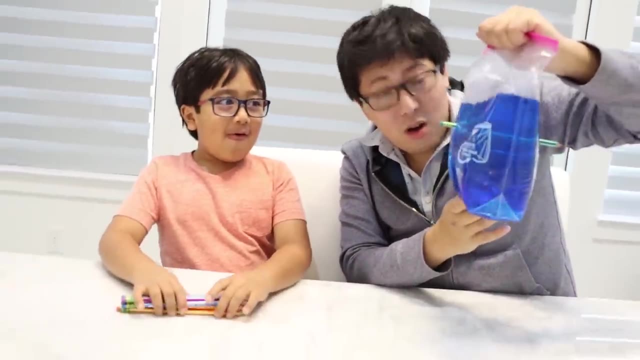 Oh, no way, guys. There's no water coming out. What? Why is it like this? How's it working, Ryan? Whoa, Do more Ryan. Okay, I'm gonna do a bunch of pencils, Whoa. 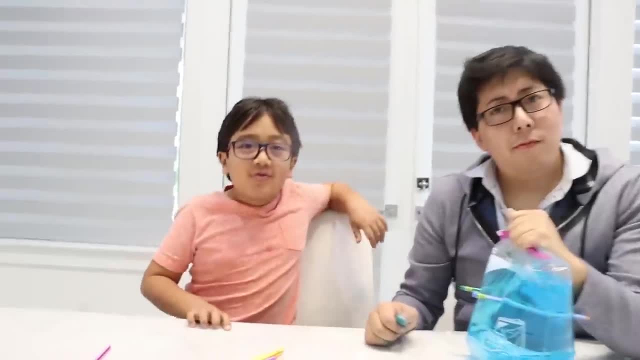 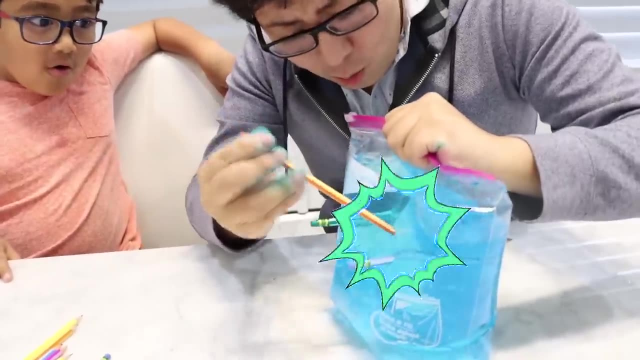 What, What, What about you try, Daddy? Eh, Ooh, can I do it? All right, let's see, I'm gonna do it at an angle. Does it work? Ooh, Whoa, it works, Whoa. 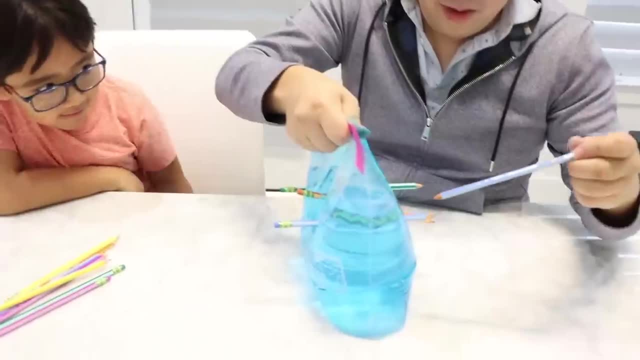 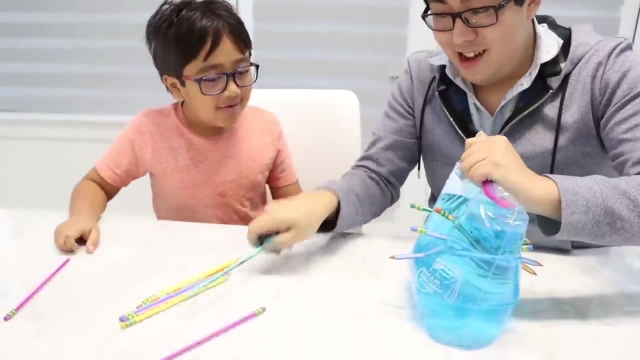 That's cool. Daddy did it from up to down. All right, I'm gonna do it from opposite direction, Up down. Whoa, Whoa, it's working. Yeah, it is Well, I'm gonna do more. 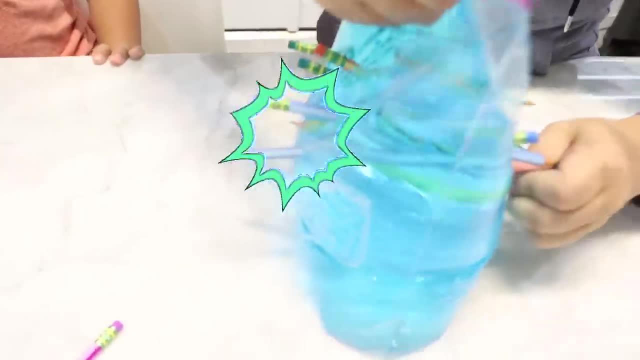 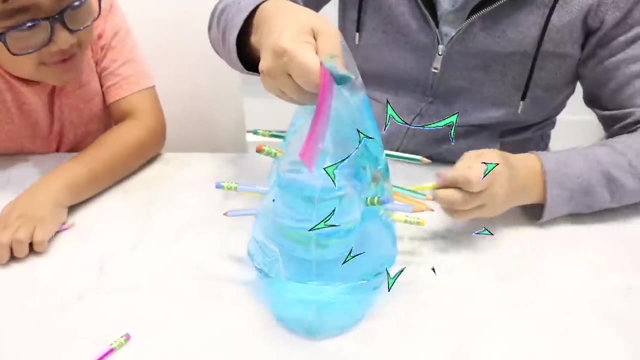 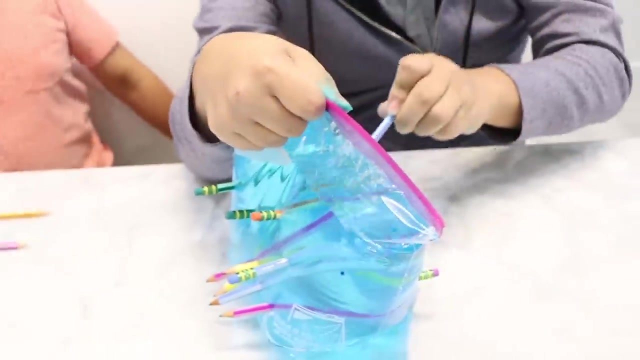 Whoa, Oh, Whoa, Whoa, Whoa. There's so many pencils, Ooh, All right, I'm gonna keep going. Woo, Woo, Let's see if I can do all of them. Whoa, Whoa. 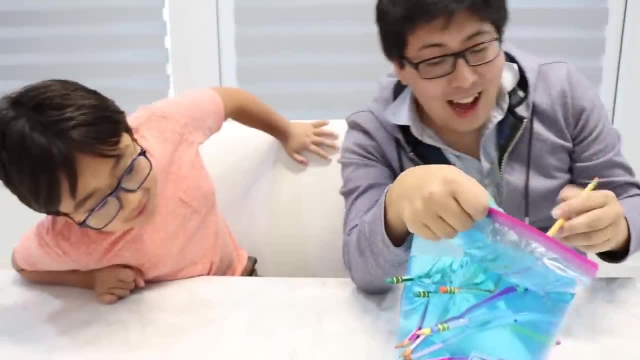 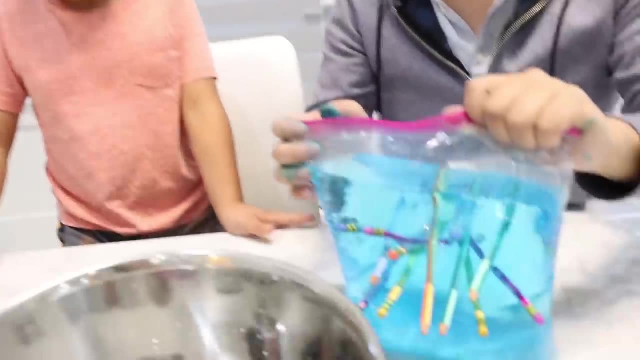 Whoa, Whoa, Whoa, Whoa, Whoa, Ah, Ah, I think I poked too much. Ah, Ah, Ah. Ah, Daddy, what about we take out all the pencils and see what happens? Ooh, good idea. 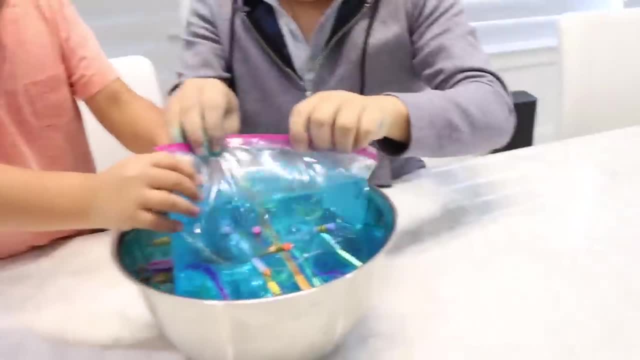 Just in case, let's put it in the bowl. all right, All right, Let's see what happens. Ooh, Ooh, Ooh, Ooh, Ooh, Whoa, Whoa, Whoa, Whoa. 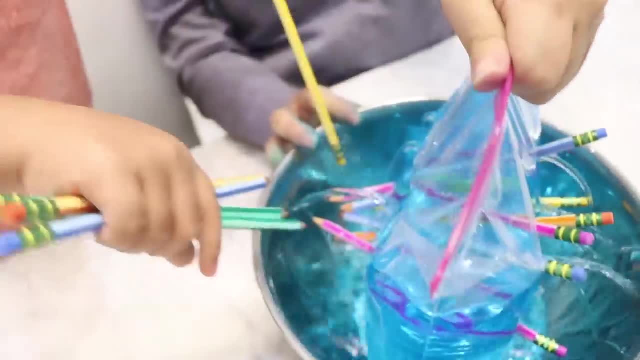 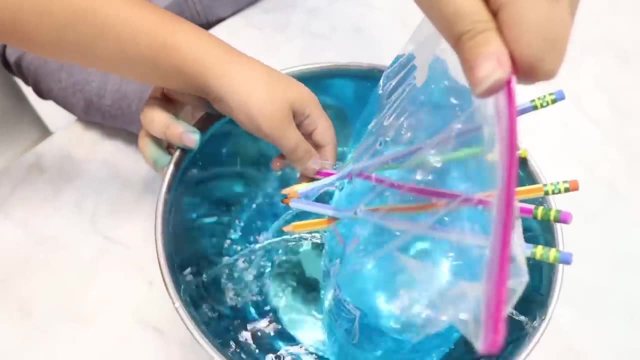 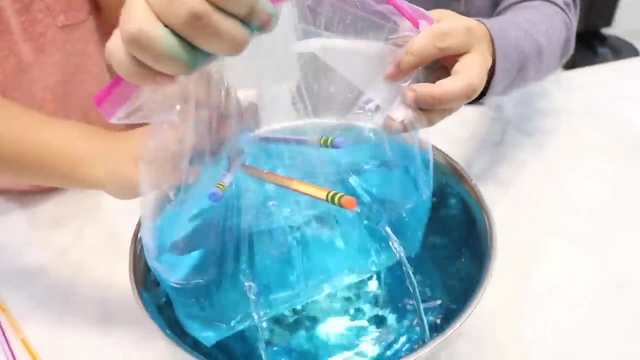 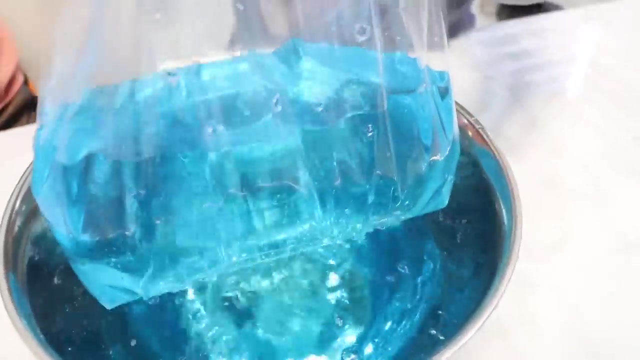 Whoa, There's so much water, Water, Waterfall, Water. those Whoa look at that. Whoa, there's so much water coming out The shower. It's a waterfall of water. Whoa, there's so much. 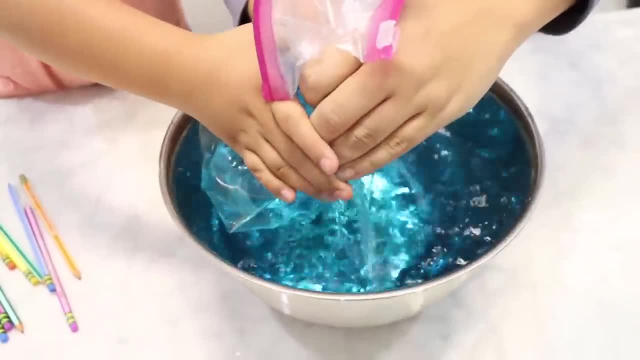 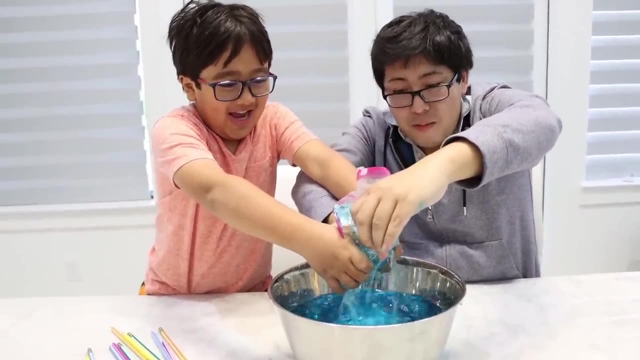 All right, I'm going to squeeze, get all the water out. Ah Ah, Whoa, Whoa, Whoa, Whoa, Whoa, Whoa, Big mess. Wow, it almost filled up the whole thing. Thank you for watching our science video about pencils. 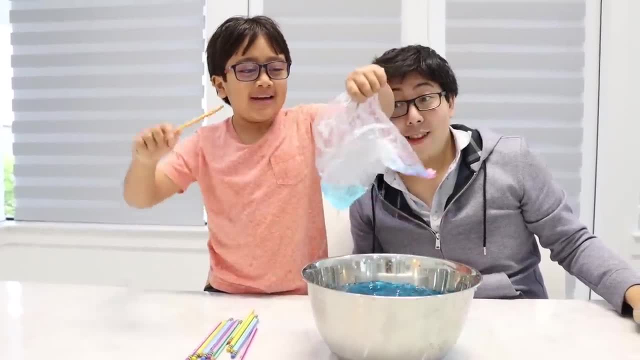 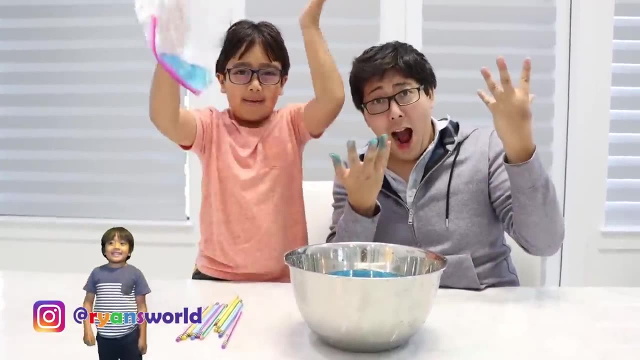 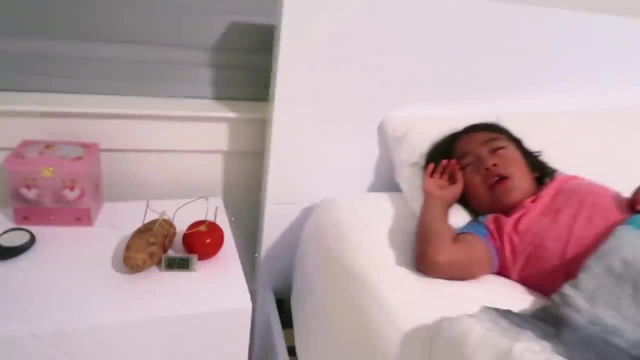 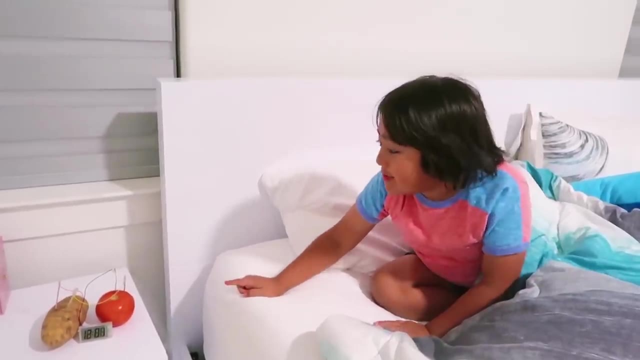 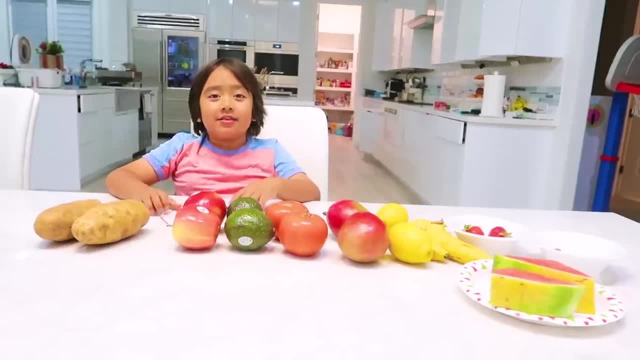 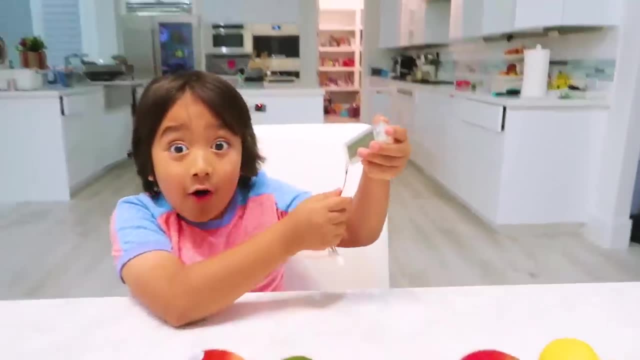 Let me show you how to make your own alarm clock. Let's go, Hi guys. So today we're going to be using 10 different vegetables or fruits and we're going to see if they can power this alarm clock. So we have potatoes. 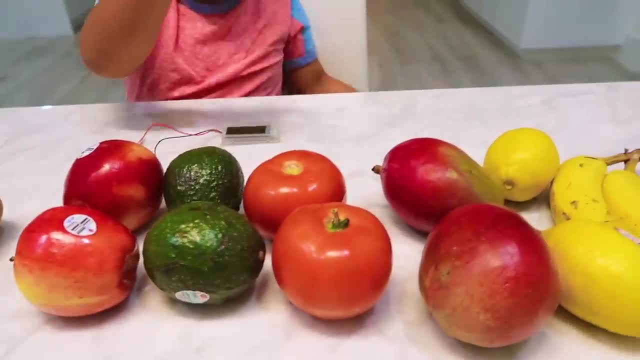 Apples, Avocados, Tomatoes, Mangoes, Lemons, Bananas, Strawberries, Grapes And watermelons. First we're going to try the classic potato. It was made for potatoes, so I think it's going to work. 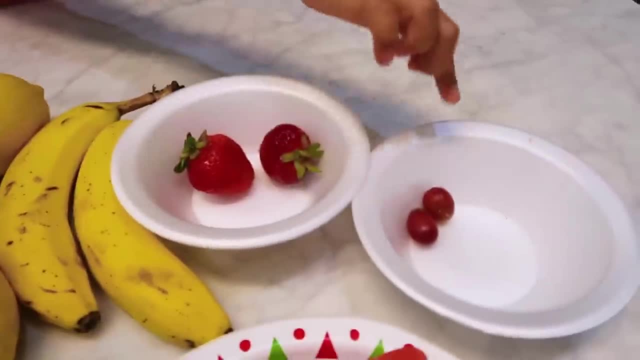 Three, two, one Oop. So if you notice here, look at the alarm clock. Is it working yet? Not yet. We got this kit online, So it comes with a magnesium water And it's going to work, And it's going to work. 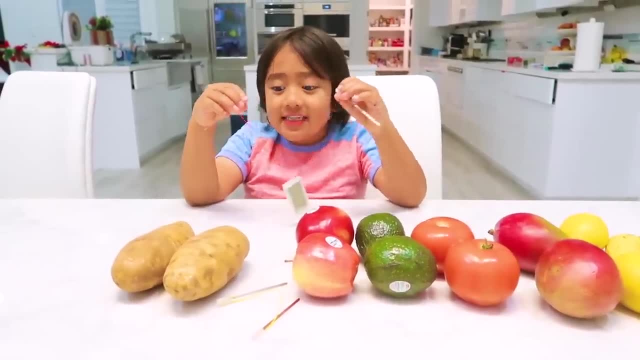 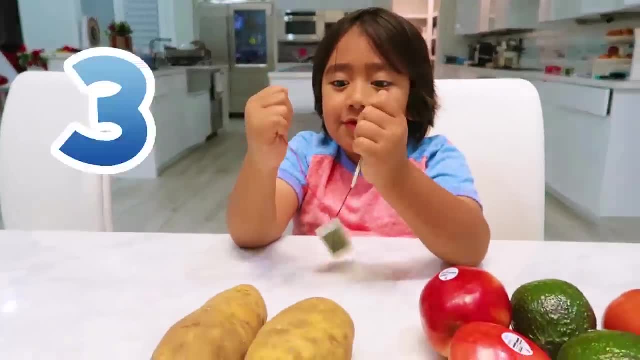 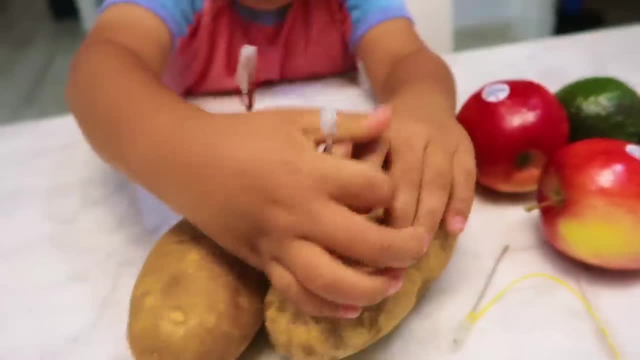 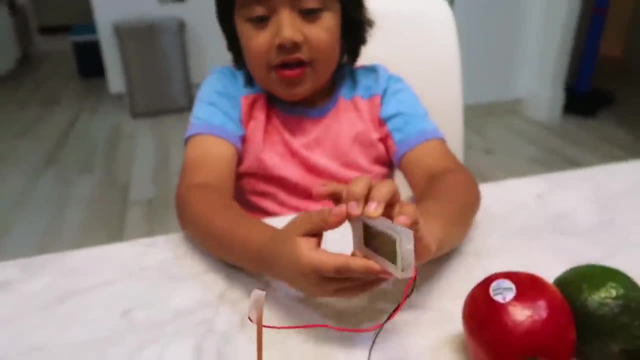 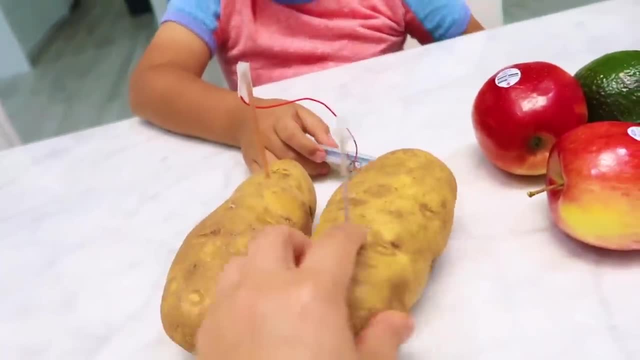 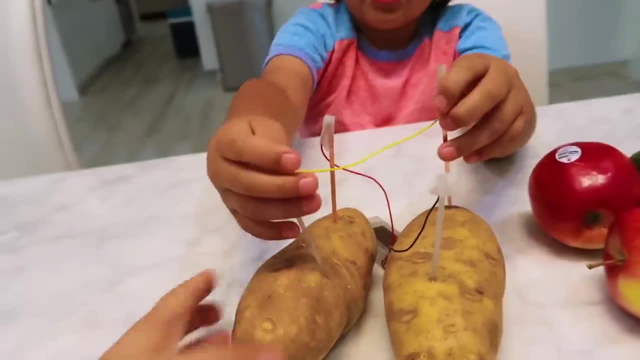 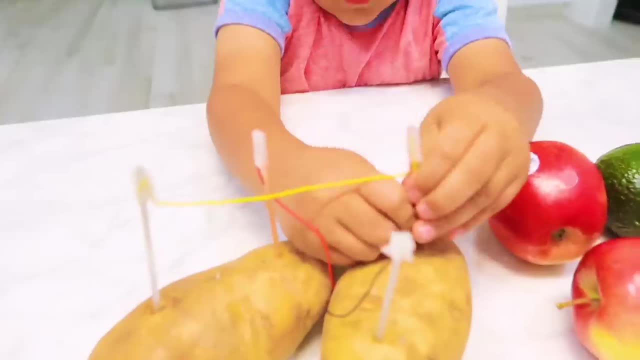 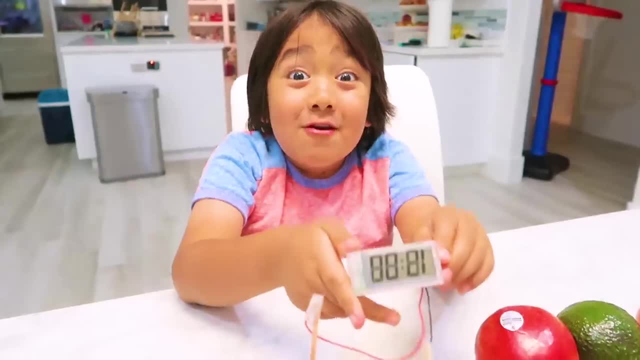 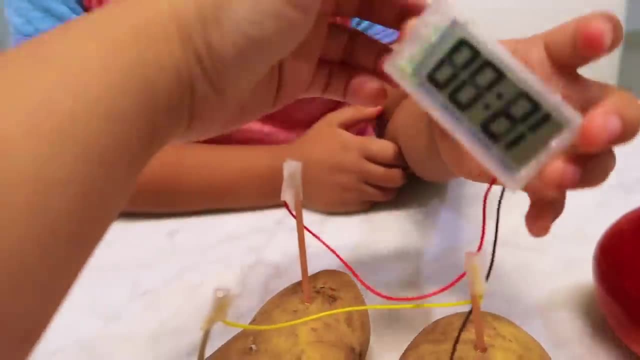 All right, you tell me, Is the alarm clock working? Look it's working. Yeah, it turns on. It's got enough energy? Yeah, So we have to manually set it. But you know, there it is, A potato works. 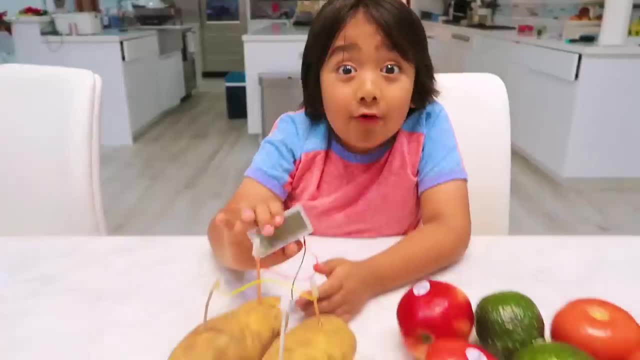 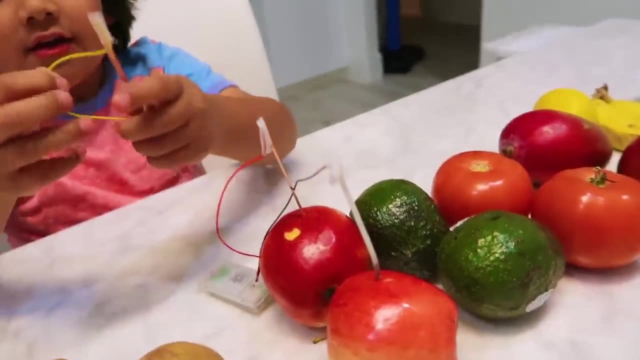 I'm going to use a potato for my alarm clock tonight. OK, Now I'll try the next one. Next I'm going to test out the apple And do the opposite on the other one. Yes, like, There you go. 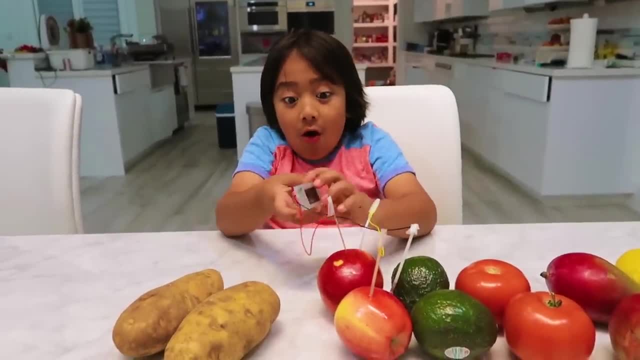 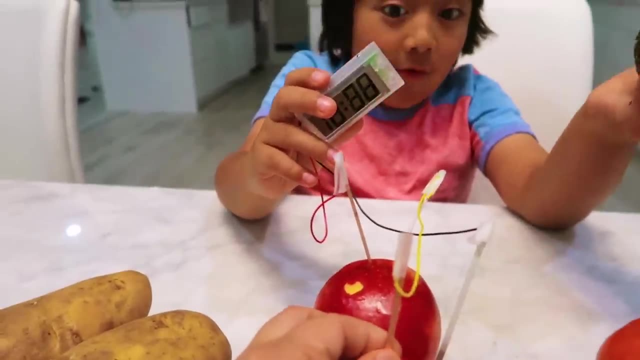 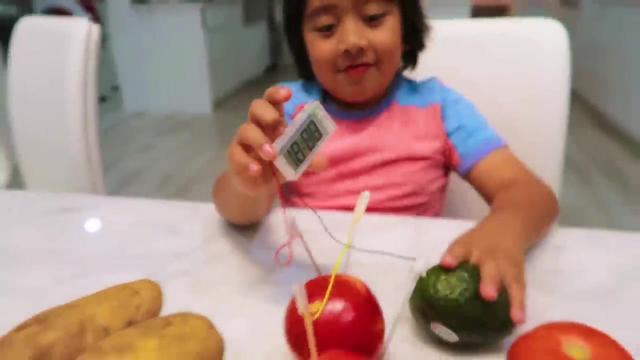 Moment of truth. Does it work? It works. Yay, so an apple can also power it on. You know it's true, because look what happened when I take out one. okay, If I take out one, it stopped working, But if I plug it back in, it works. 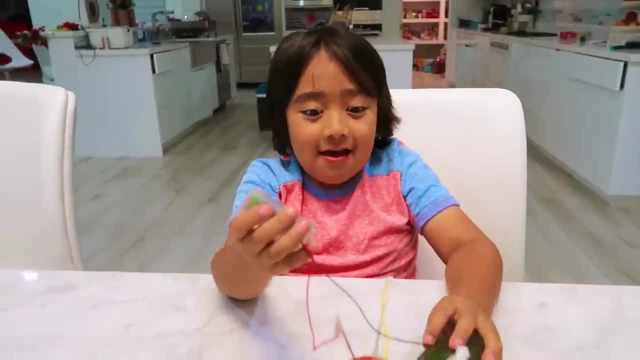 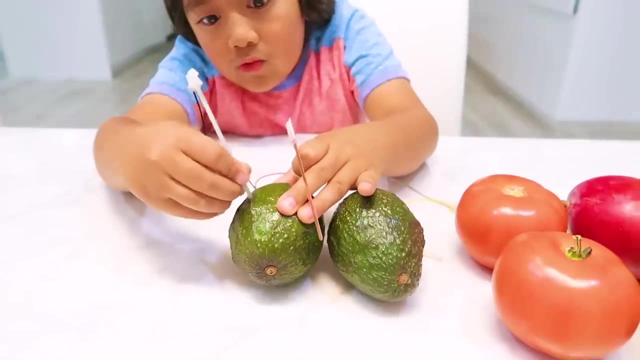 I'm really interested for this one: The avocado Guys, let us know if you think avocado can power on the alarm clock. Now we're gonna try the avocado. Ooh, ooh, ooh, ooh, ooh What. 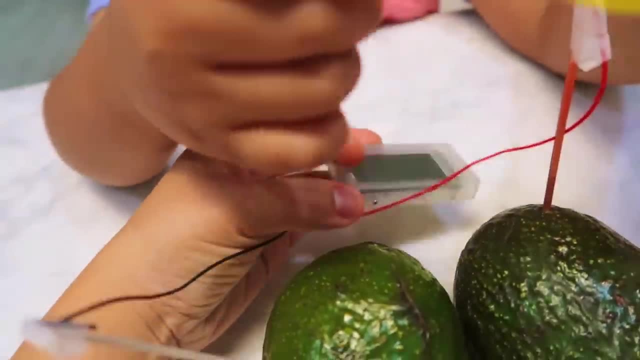 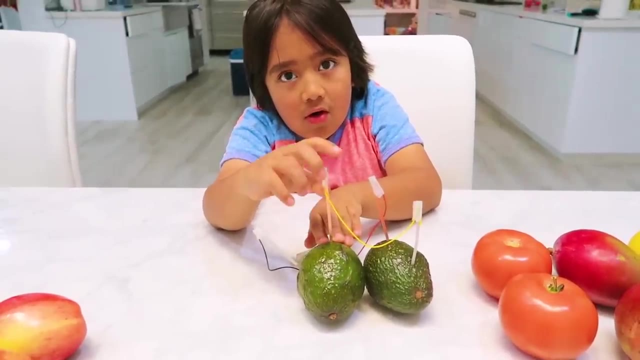 Oh, I think it's gonna work. You think so. Yeah, You guys notice right now nothing's on right, So it doesn't work right now. So Ryan's gonna put it in. Can you use an avocado alarm clock tonight? 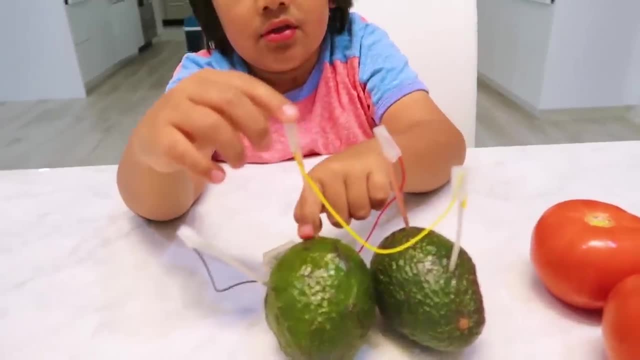 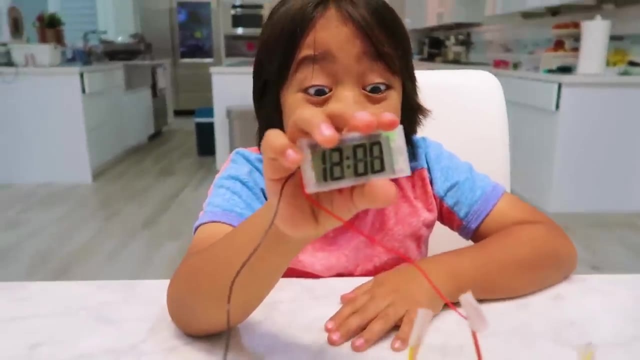 Wait, what did I say? I don't what You're supposed to put this. No, that's right. yeah, it's supposed to be opposite. You need that to complete a circuit. Does it work? Avocado work. 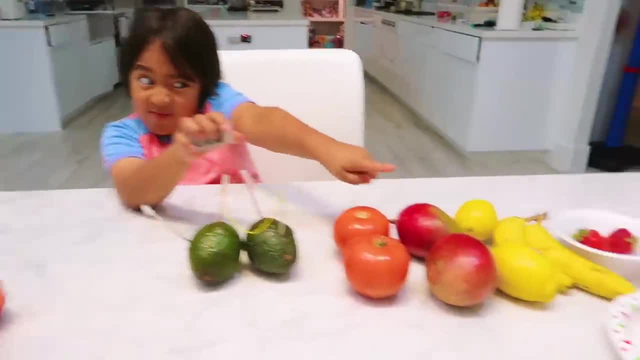 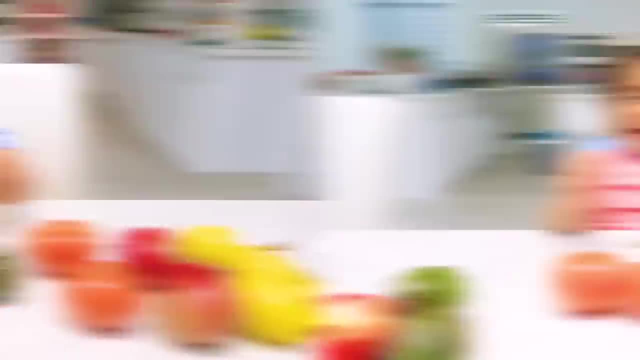 Whoa. Now the most interesting part. The most interesting one is one, That's true, That one we're not sure. Also, tomato, Wait, no, I think tomato will work, Tomato will work. Okay, let's see. Now we're gonna try tomatoes. they're really messy. 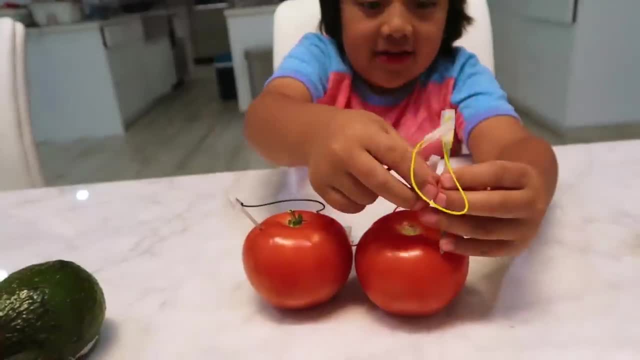 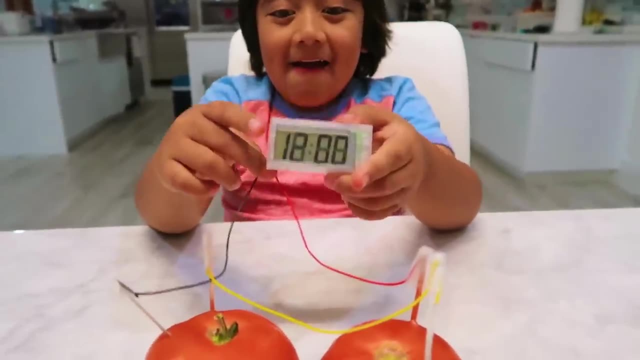 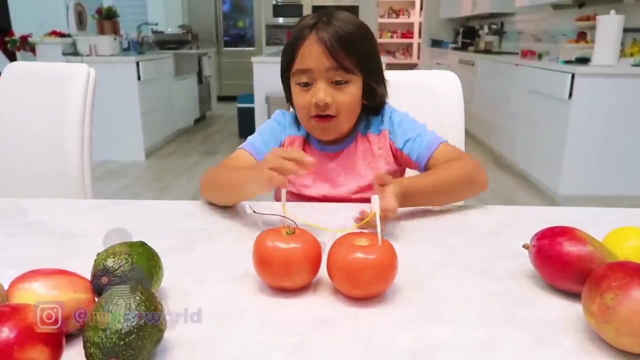 Don't poke it too hard, I don't know. Pop And like this. Does it work? It works, It does work. wow, Maybe we do need just fruits and vegetables To power our alarm clocks. You think fruits and vegetables work? 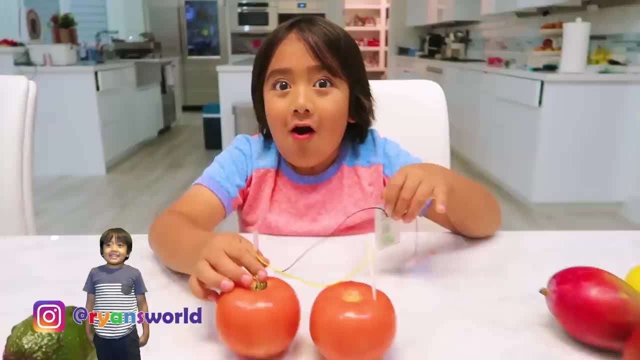 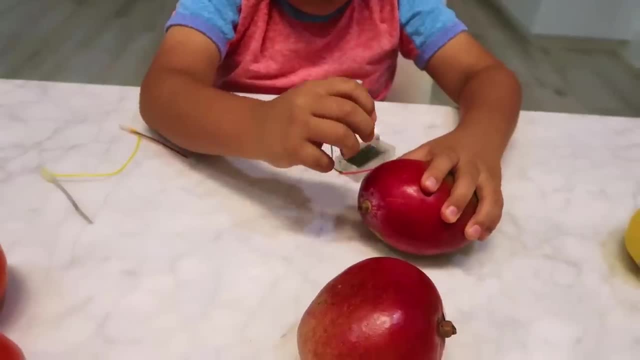 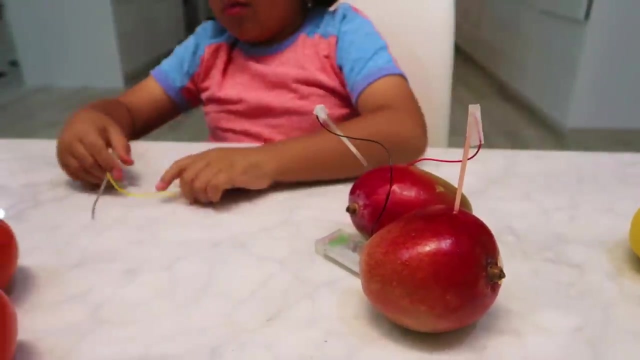 Fruit and vegetables can power on your iPad. That's a fun experiment to do later. Ooh, Okay, now let's try mango. Oh, it's bending the wire Here And then one, So you need the other part to make like a circle. 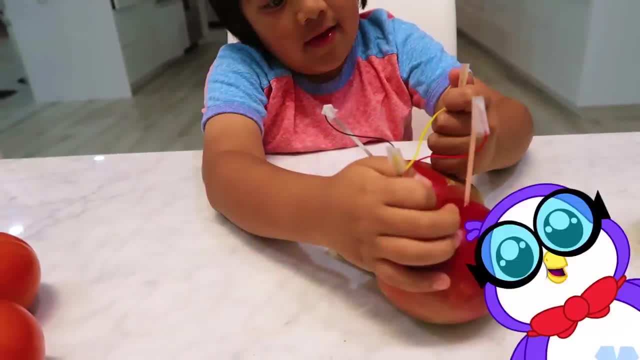 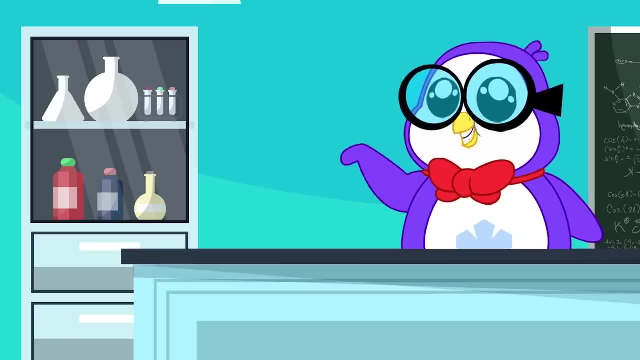 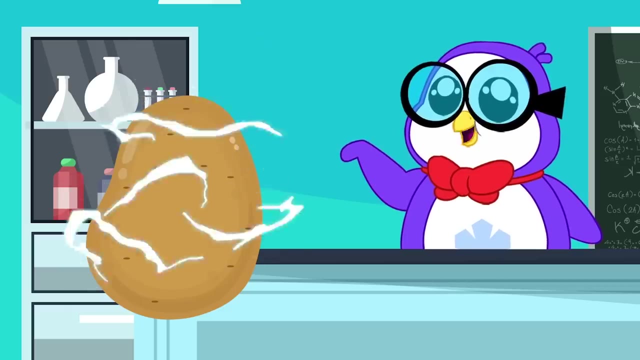 You have to complete the circuit. that's why you need it. Actually, the potato clock works by converting chemical energy into electrical energy. Did you know that the energy doesn't actually come from the potato, but rather the energy comes from the metal dissolving inside the potato? 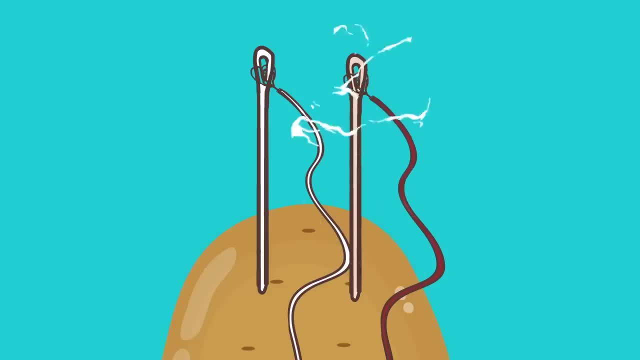 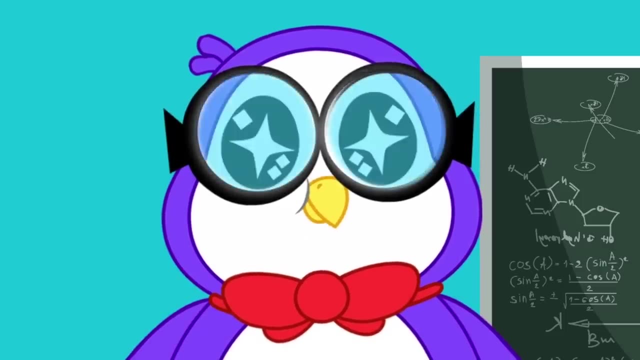 The energy made from the reaction moves to the copper, strip down the wire and into the clock, making the clock turn on. That's spectacular. Yeah, Wow, everything worked so far. look, Yeah, Which one do you wanna try next? 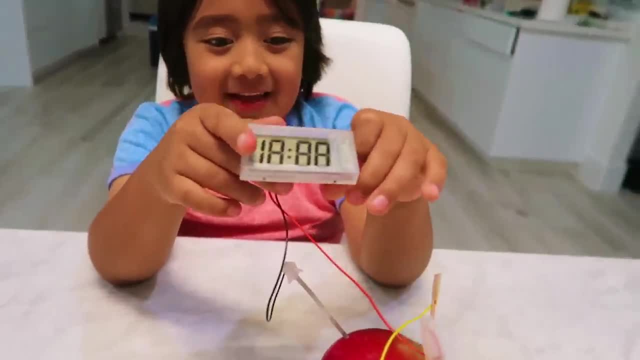 I wanna try the banana. The banana, Wow, that's interesting. I think it'll work. You think so. I think it has energy. Now let's try banana. I'll try it like this. Okay, So it's easier to do positive than negative. 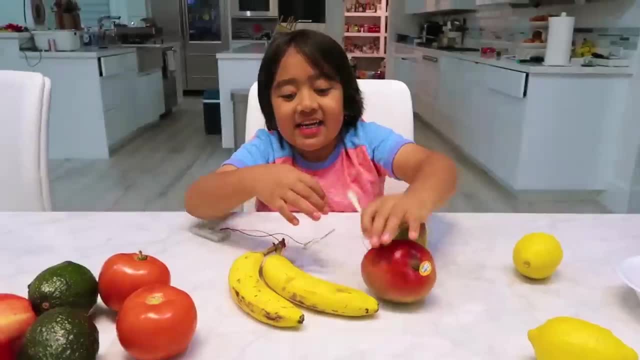 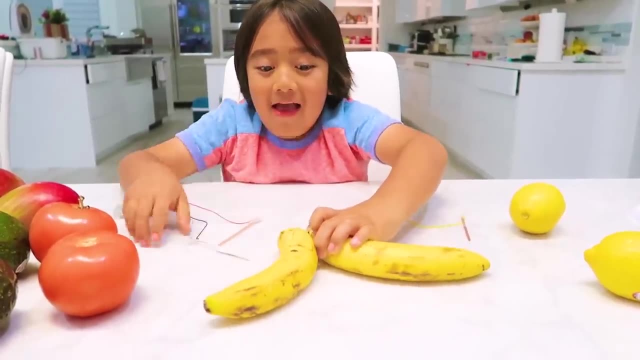 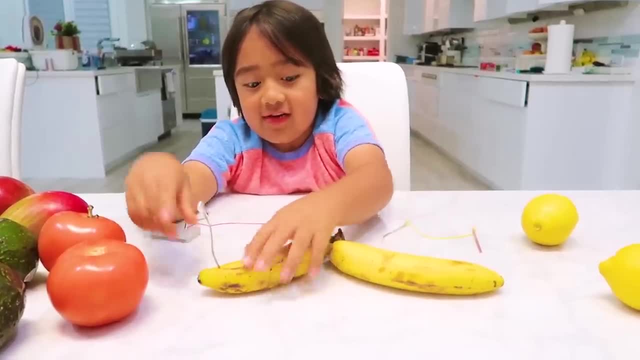 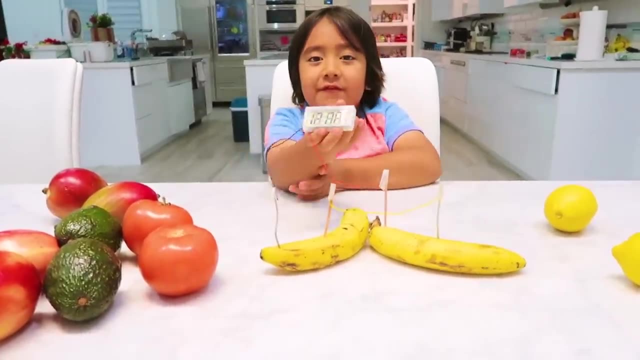 I'm not, I'm not, I'm not. Yeah, if it tastes well, I'll put it here. Yeah, put it anywhere you like, Well, Enjoying a different time, but yeah, Oh, it does work, yay. 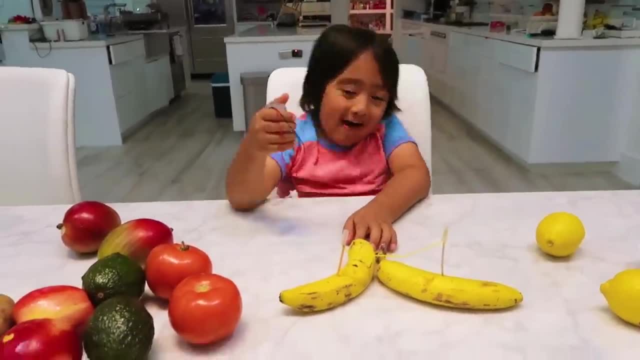 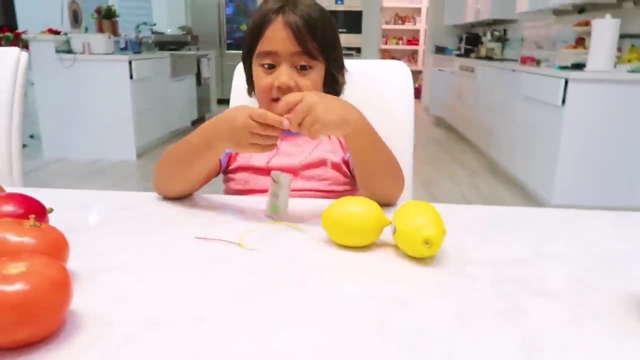 You can have a banana clock, Woo-hoo. Now let's try Banana Whoa. What do you think, Ryan? The lemon's gonna work. Yeah, I think so. Oh, yeah, it's gonna work. It's hard to poke in. 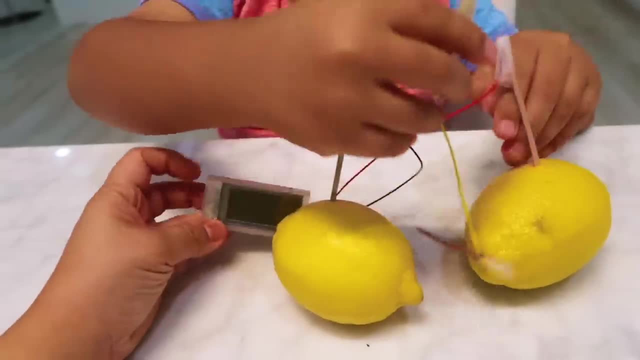 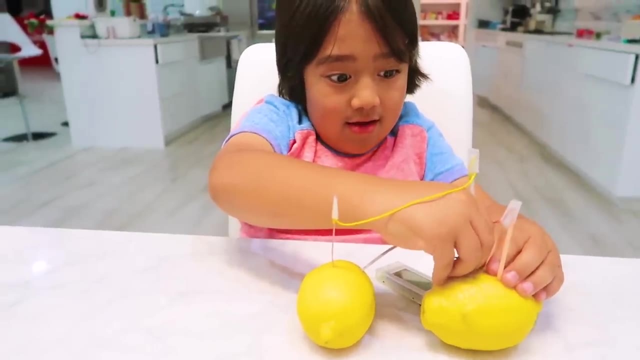 It kinda has a smell. See, right now it is not on you guys. Three, two, one. What do you think it's gonna do? work or not? Definitely work. I don't even have to poke it in. 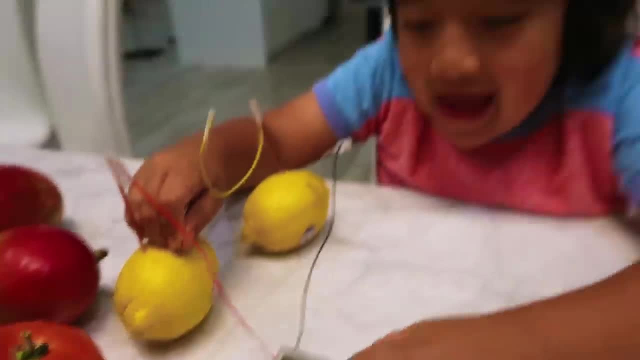 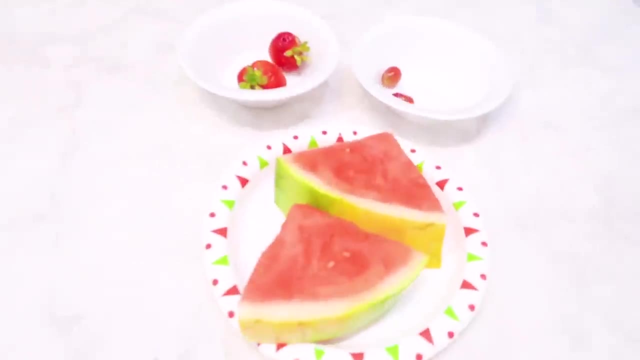 What. That's crazy. So I guess you don't really need a lot of power, But so far everything works so far. Which one do you wanna try next? These three, I'm very interested. Yeah, I'm gonna try this one. 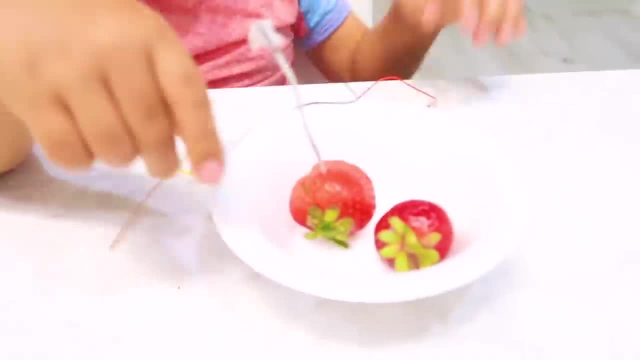 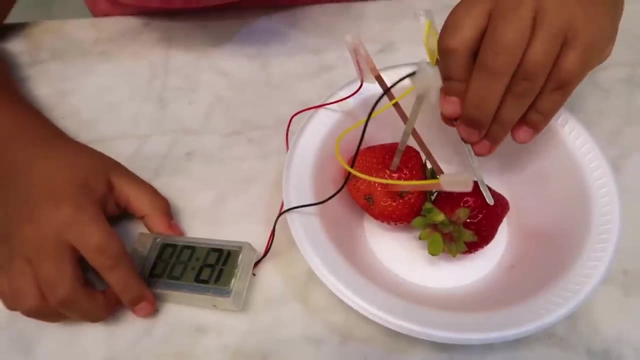 Strawberry, Strawberry. You barely have to poke this in. to poke it in, I'm gonna see if we can do the same thing we did with the lemon. Oh, good idea. Look, look at it. Wow, very cool. Which one do you wanna do, Ryan? 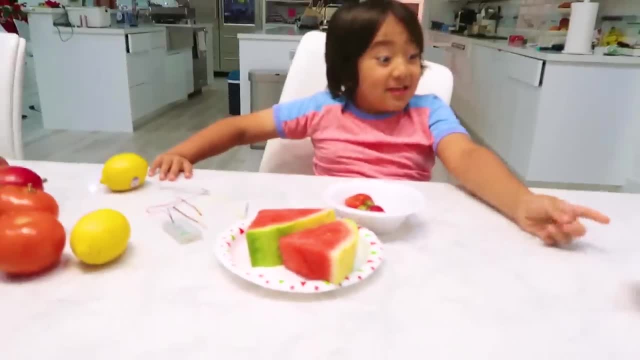 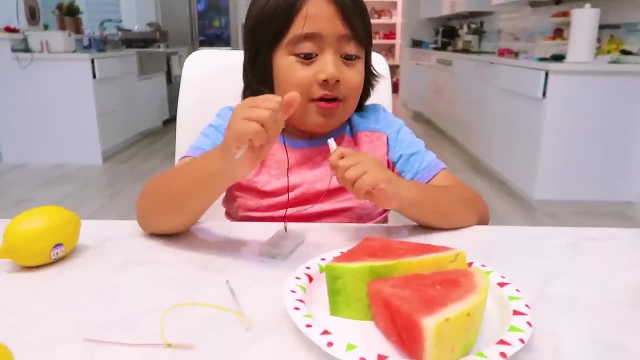 Grapes or watermelon. Watermelon, Okay, because grapes it's so small, I know. Is it gonna work, Because it's so tiny? You think watermelon's gonna work, Let's see. Okay, Oh, it's so easy to poke in. 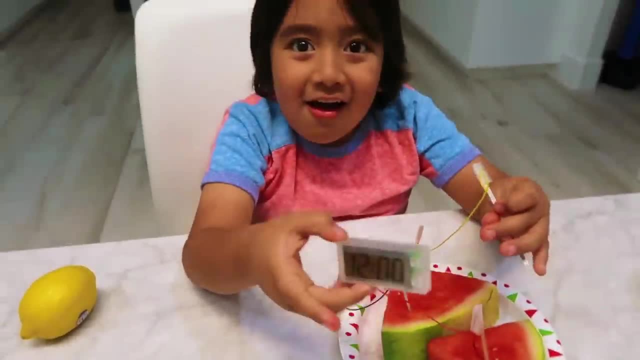 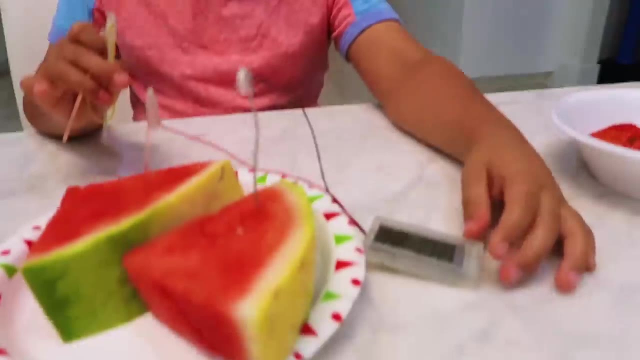 Yeah, What Is it working? What Guys? I didn't even need to complete the circuit, It just powers off with two. Wow, I didn't know watermelon's so powerful, But this makes it a lot more powerful, So it does work. 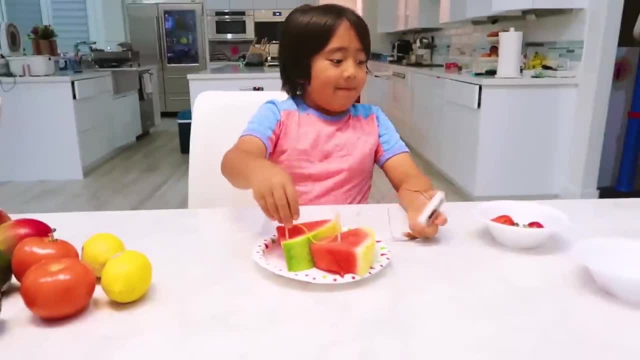 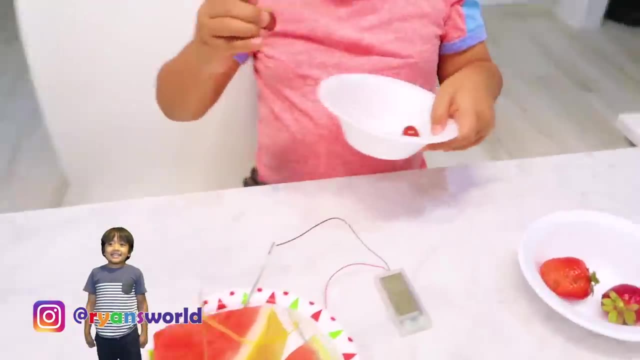 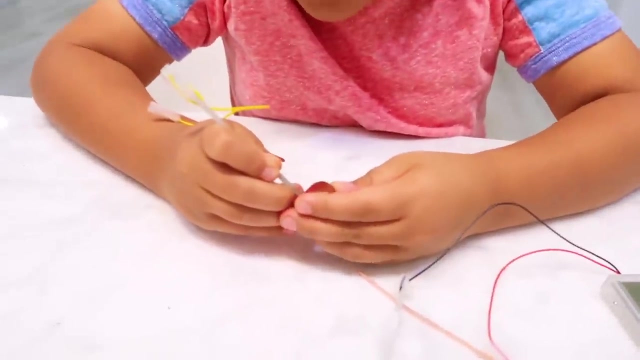 Yay, Yeah, Let's try the last one in the most. Wait, how is this gonna work? I don't know. It's so small. I did positive. You have to stick them very gently, Can you do it? 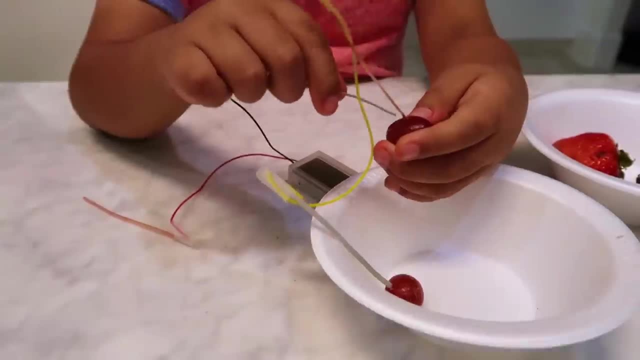 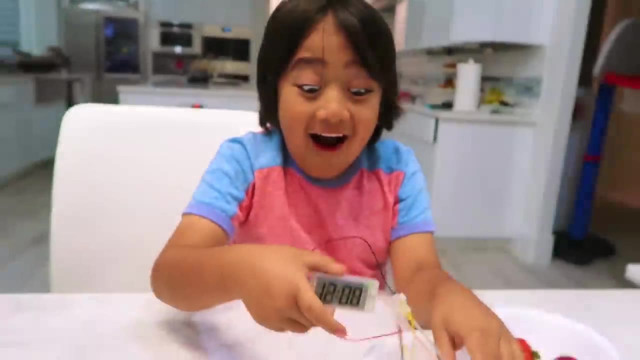 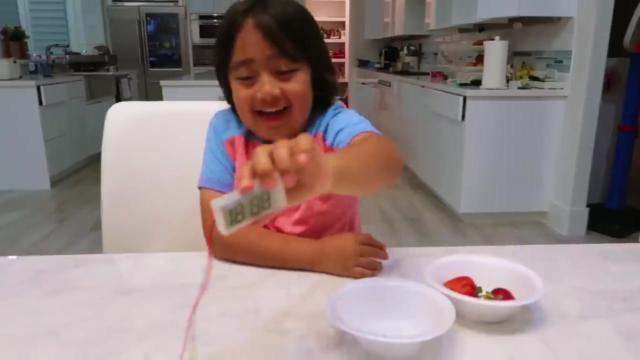 Yeah, I did one. Now I do the other one. So far it's not working. Let's see What Grapes can power on a clock. Look at that, you guys. Just two grapes, That's it. You don't need two grapes. 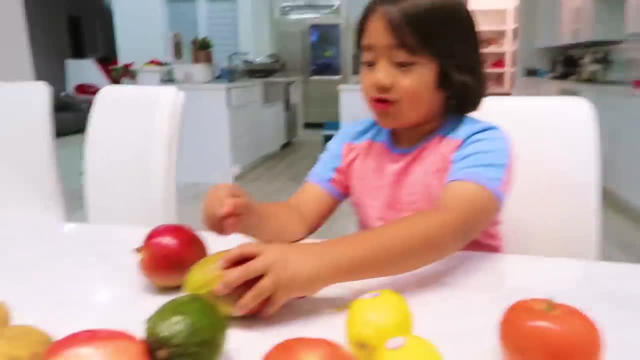 Don't need a whole potato, You just need two grapes. Well, what if you just try one of them? Yeah, With all of them, It's working. Yeah, all you need is one fruit, One grape. it is, It does work. 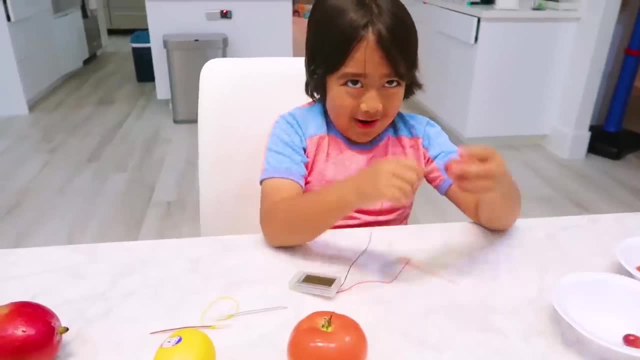 Look, Just one too. We don't even need to complete the circuit, It's so powerful. This is the most powerful. Yeah, I think all you need is one, Ryan Like this. So Ryan's trying out different ones. 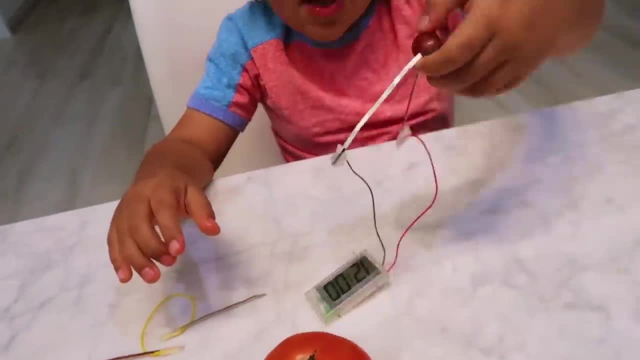 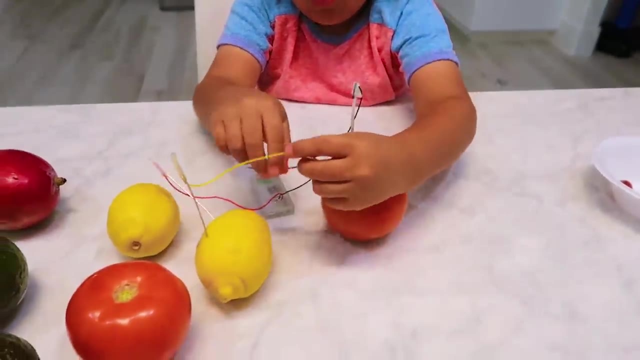 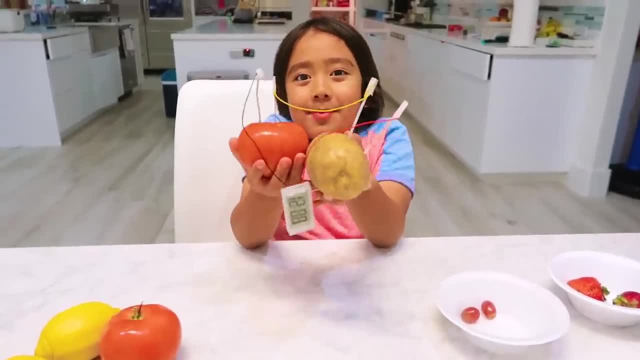 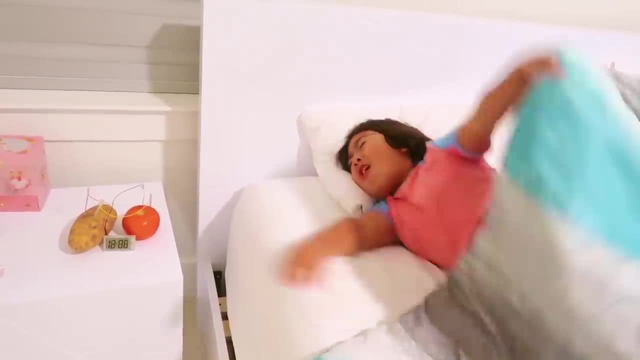 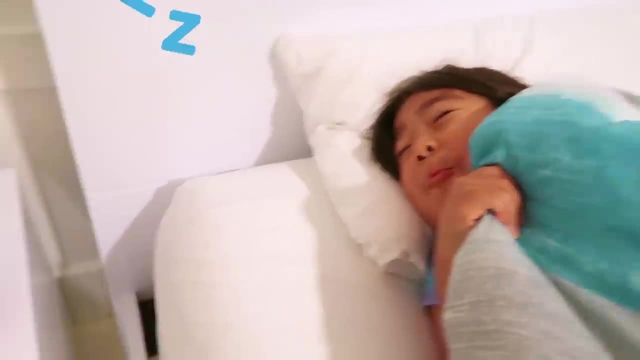 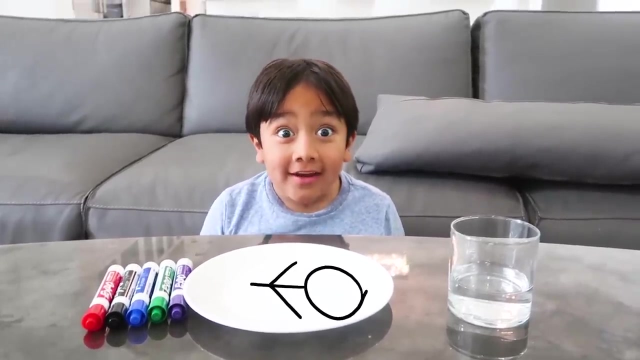 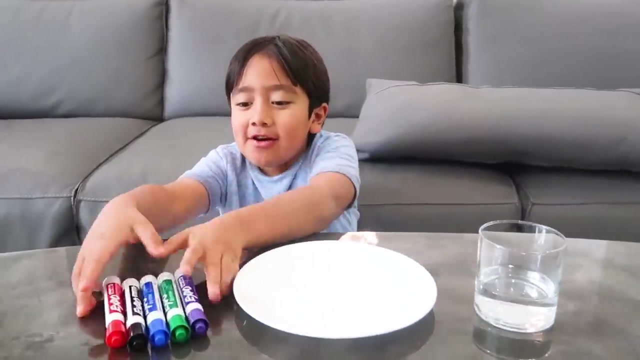 And that's how you make a fruit and vegetable alarm clock. Bye, Hi guys. Today we're going to put our trolley- Yeah, we're going to put our trolley- with a red eye out- Okay, Wow, and then make it float on water. so this is very easy. all you need are some 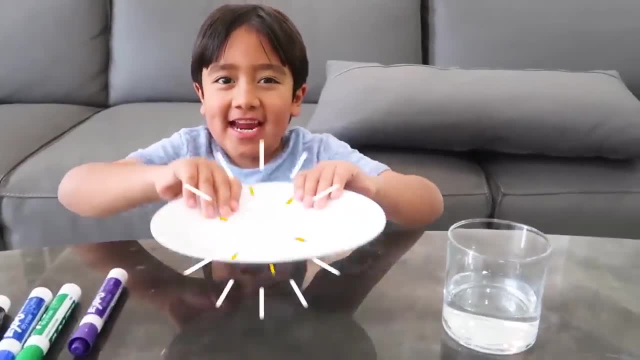 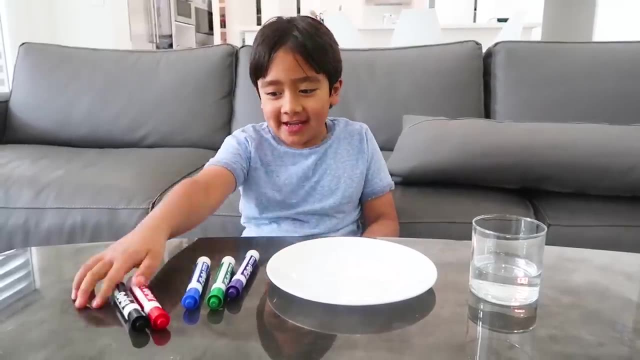 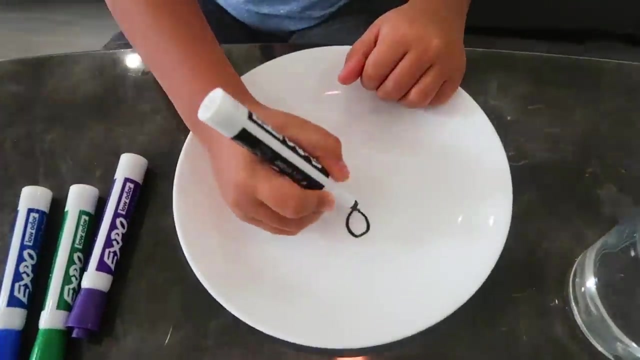 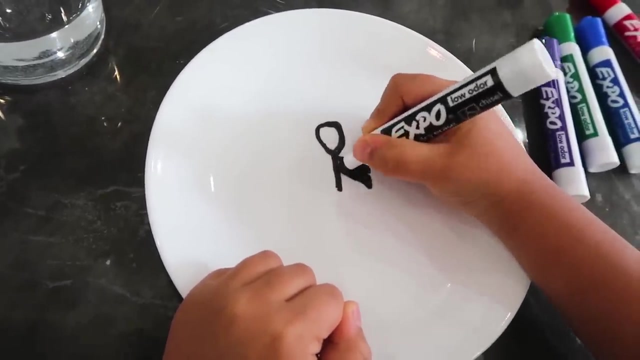 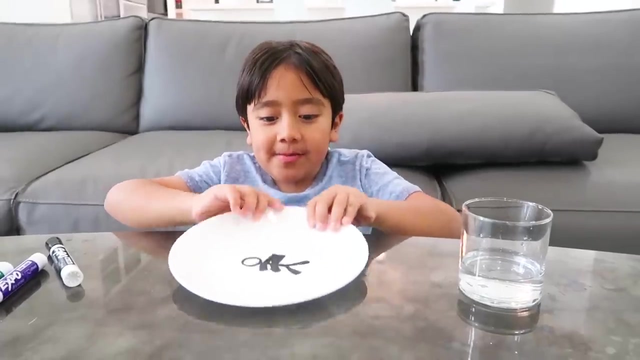 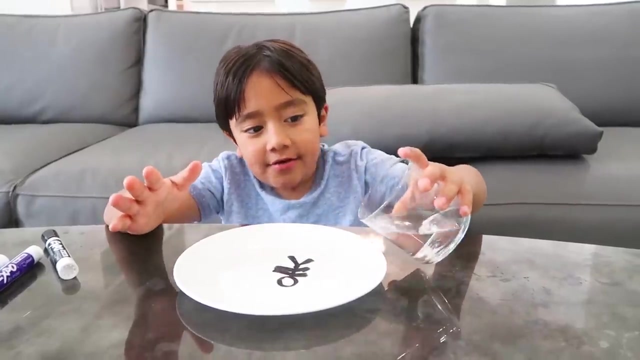 markers, a plate and some warm water. first draw what you want on the plate. well, I'm gonna make stick figures with multiple arms, what so? like this, make it really thick. you make arms and then you make the legs. so after you make your drawing, then you put some warm water on this side. 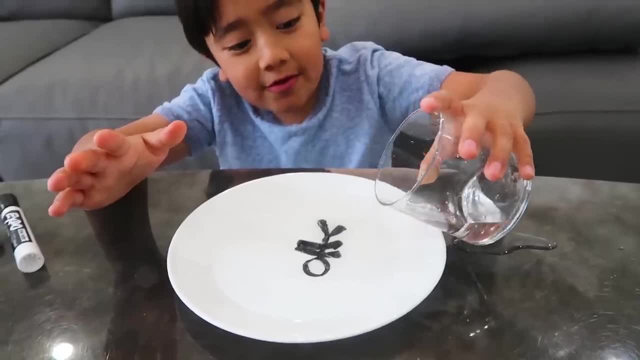 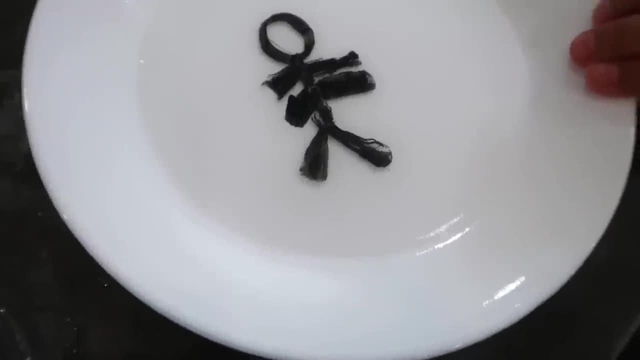 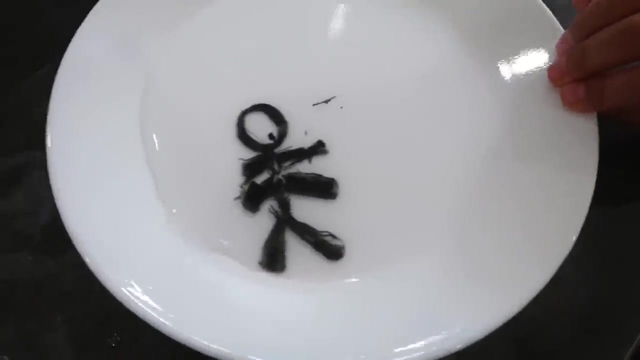 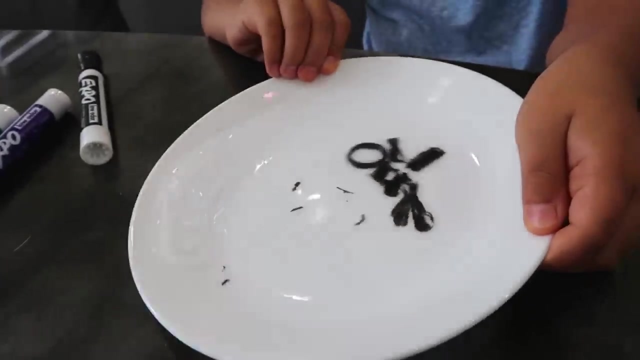 whoa, you move. look he's dancing. oh, you don't sue. oh, I feel like the arms or legs gonna break. oh, it's moving now. yeah, now you can just walk. dude, daddy, daddy, daddy. this is easy way to make your stick think you're float. he broke this. 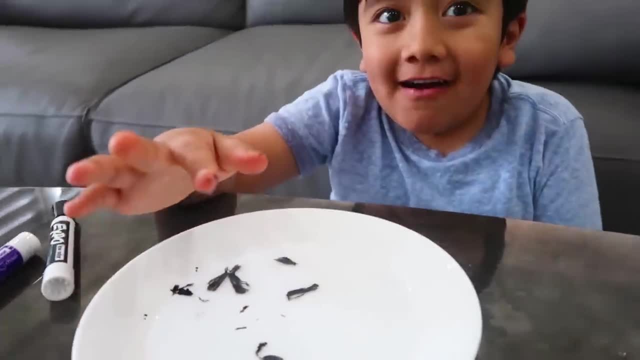 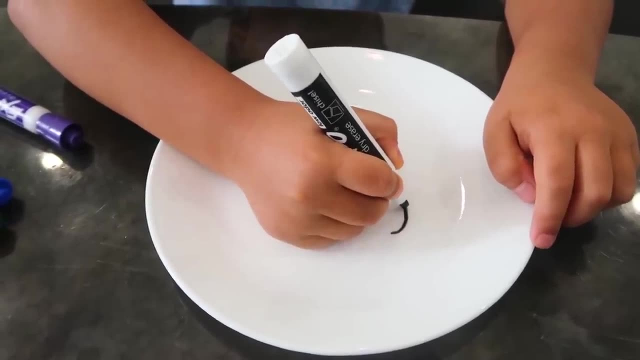 is easy way to make a stick figure. float he broke. this is easy way to make. This is so cool You can hold it. Okay, guys, for the next one I'm gonna make a dog. It should be like this, And then maybe I can put like ears. 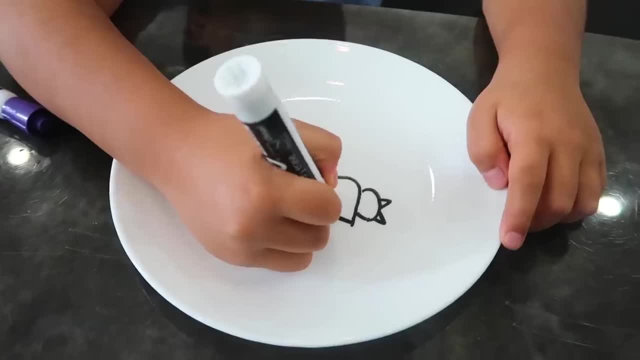 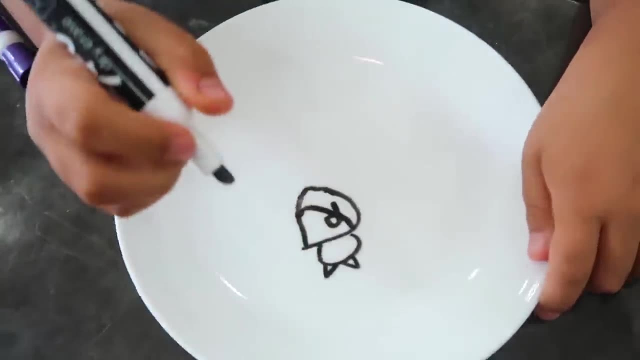 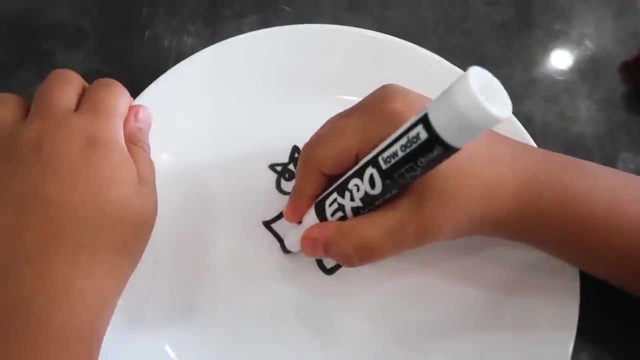 I feel like I'm making a cat. I'm making a big dog or cat. Oh, I can't do it right, Unless I do, like this, I put an R. Okay, then I'll make the legs and then the arms. 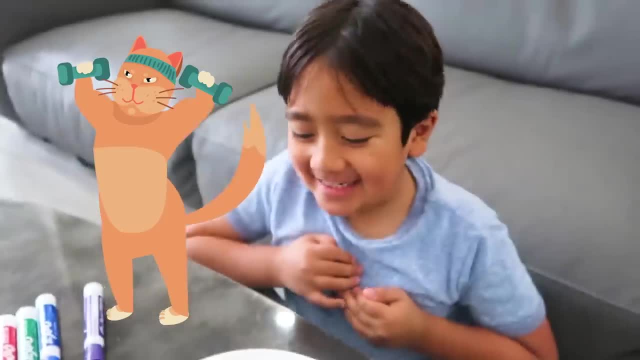 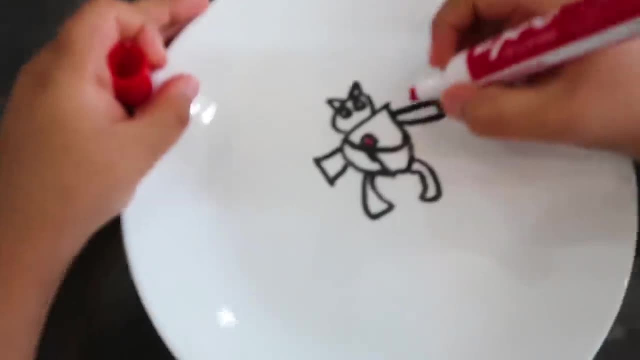 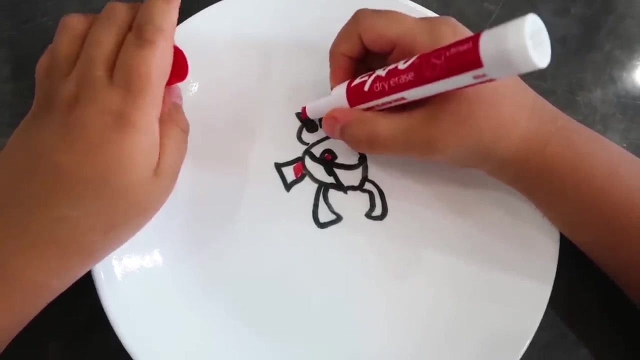 I feel like I'm making like a super strong cat or something Meow. Okay, now I'm going to put red right here And then I'm gonna make this red, And then I'll make the eyes red On the ears. 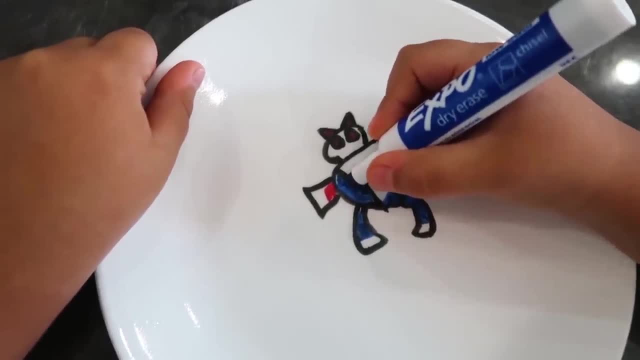 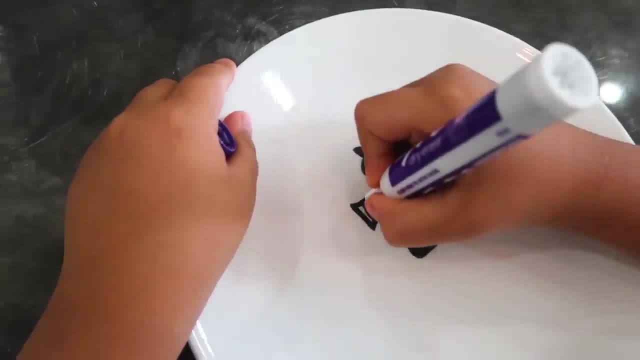 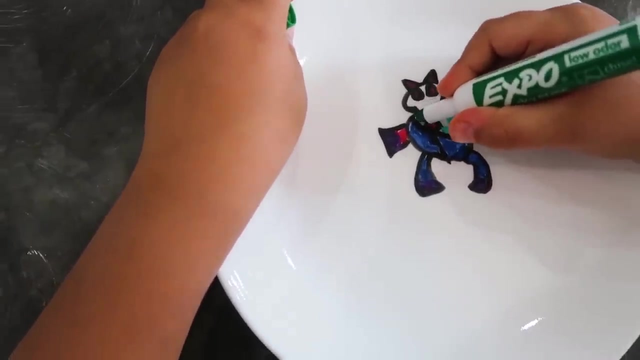 Okay, so I'm coloring the pants. He has jeans. Okay, I'm gonna make the skin color Purple. Okay, I'm gonna put it here And I'm gonna put this part green. Okay, like this And Perfect.